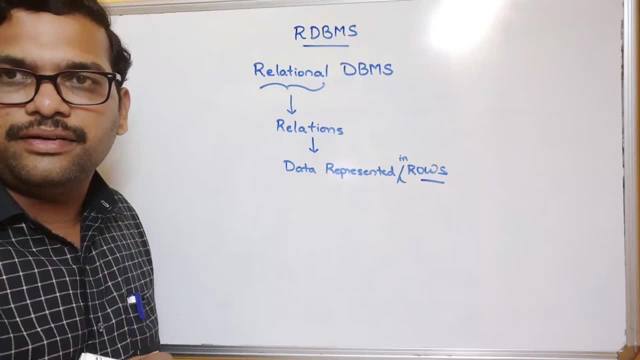 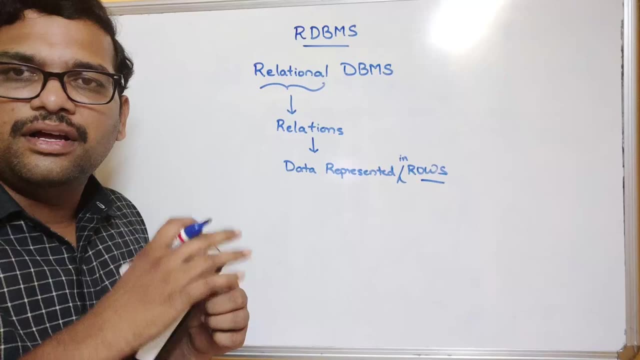 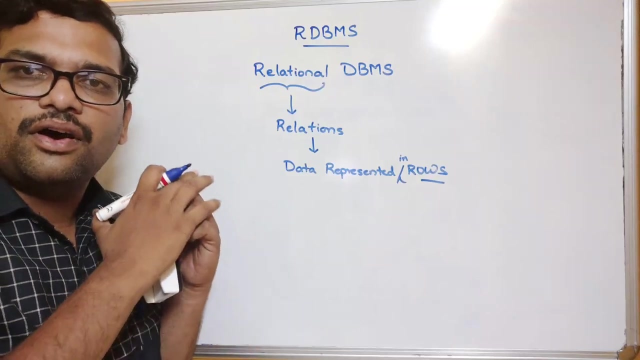 tables will be very easy to access the data. right? If any sort of the data is organized in the form of tables, then automatically it will be very easy for accessing that particular data. So that is why. so this is a relational database and modern softwares will be using. 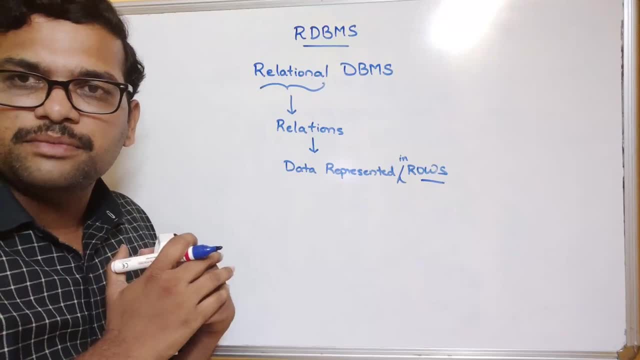 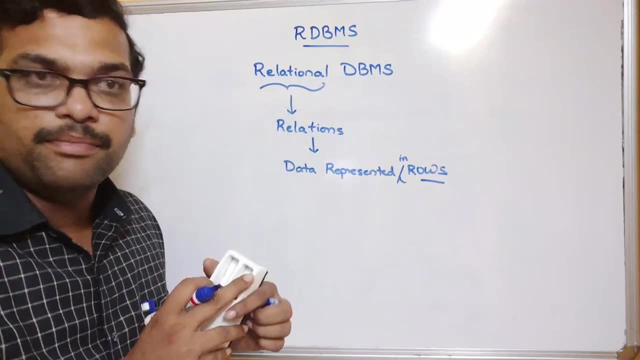 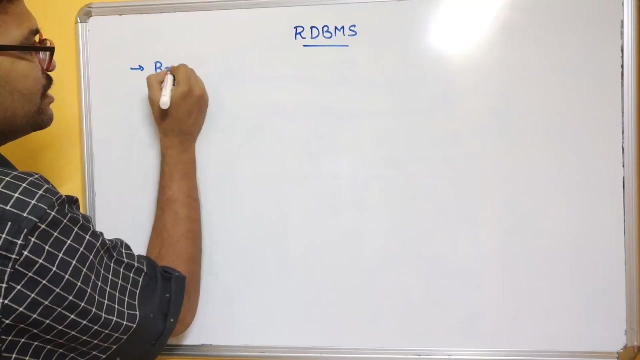 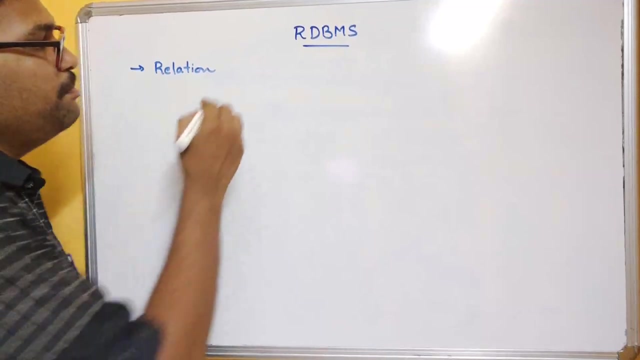 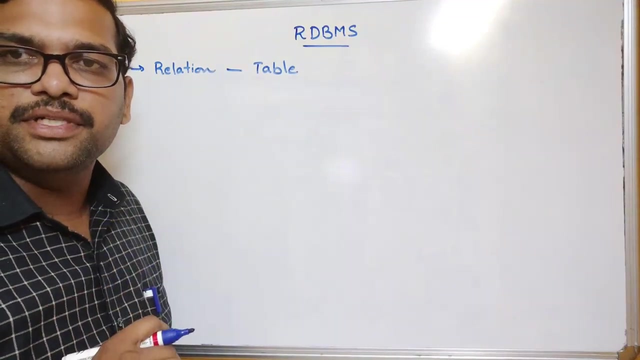 related to this relational database management system, that is, a relational DBMS, RDBMS. Now let us see what is RDBMS. So the first one is a relation. So what is meant by this relation in RDBMS? So this relation means table. Table is also known as a relation in RDBMS, For example. 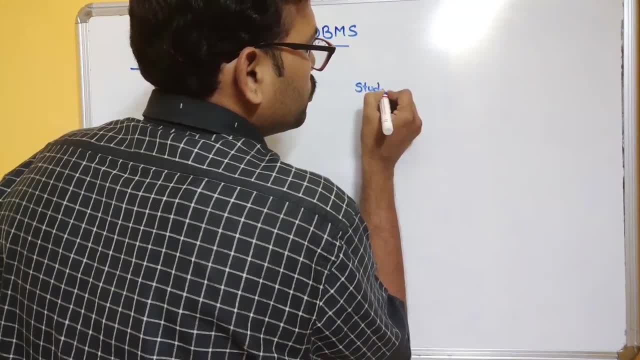 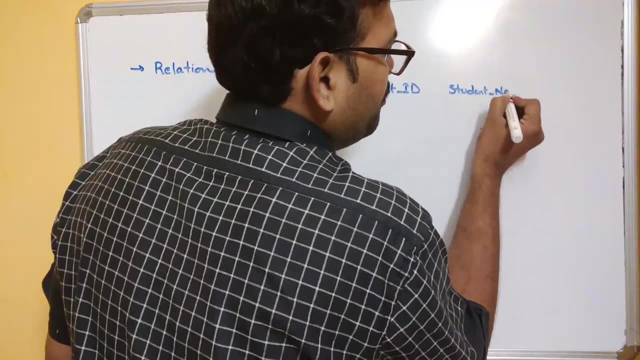 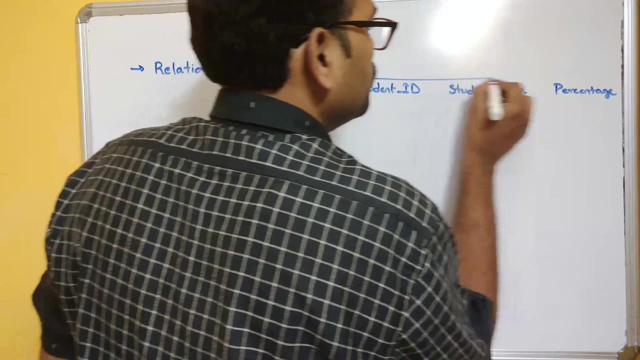 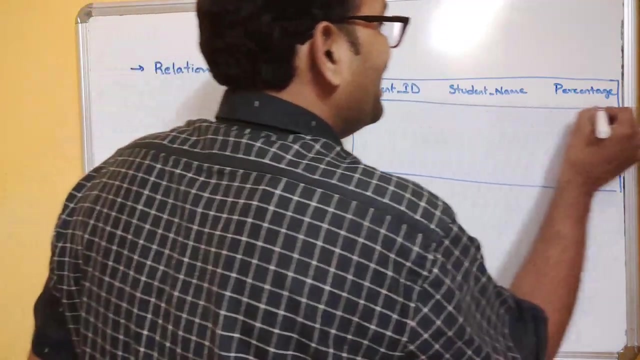 consider the student database. So student table, So student ID, So student ID, So student name, student name, student name, percentage percentage. So this is the table. This is called a table or a relation. It's called a relation. For example, student number is: 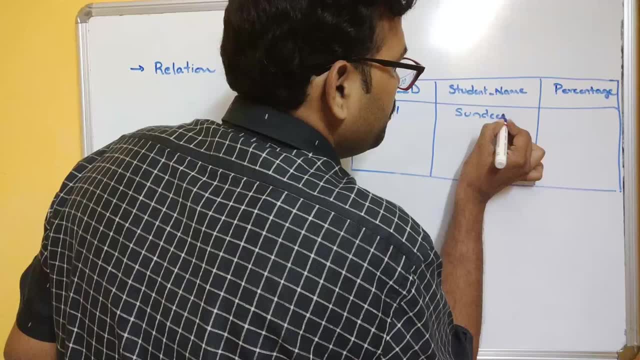 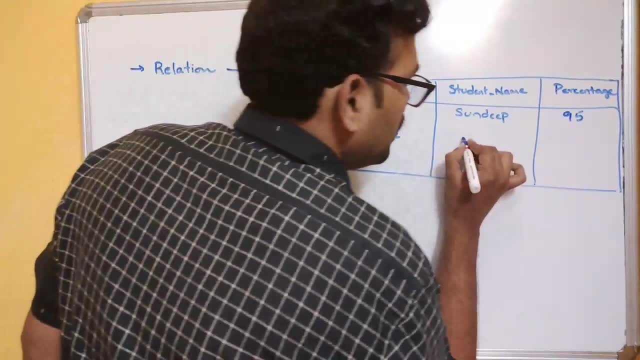 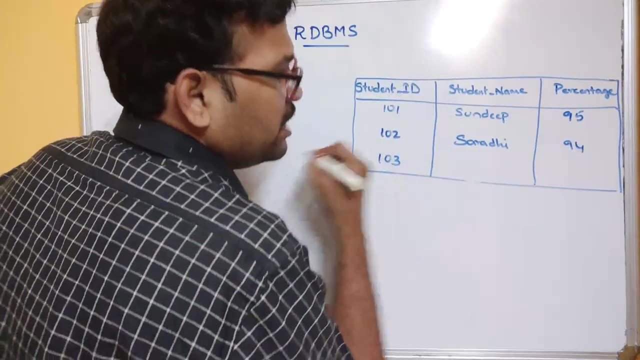 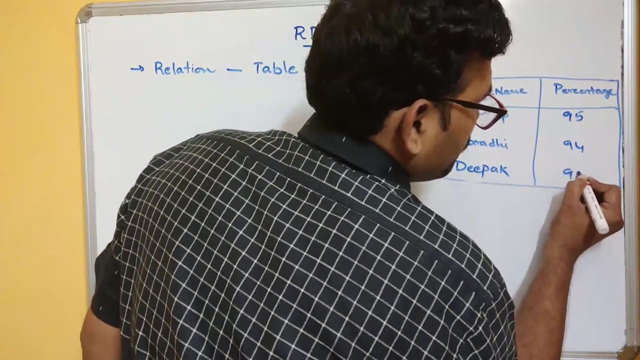 one at one and the student name is some Sunday and the percentage is some 95 and the date number is 102 and name is Samsaradi and some percentage is 94 and 103. the student name is some Deepak and the percentage is some 90,. right, So this is the student table. This is a student. 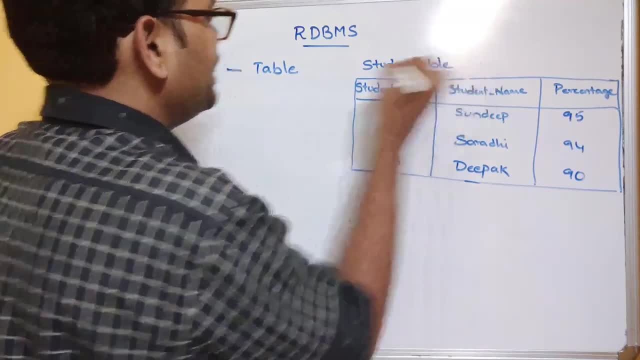 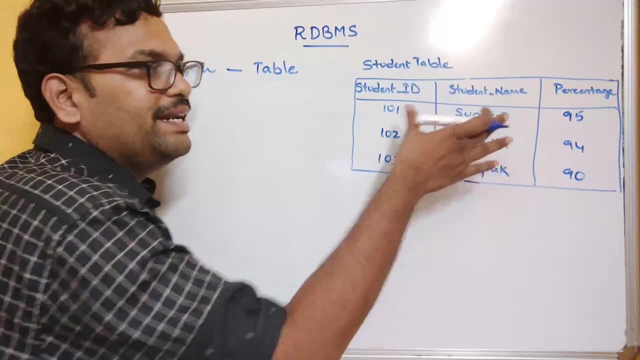 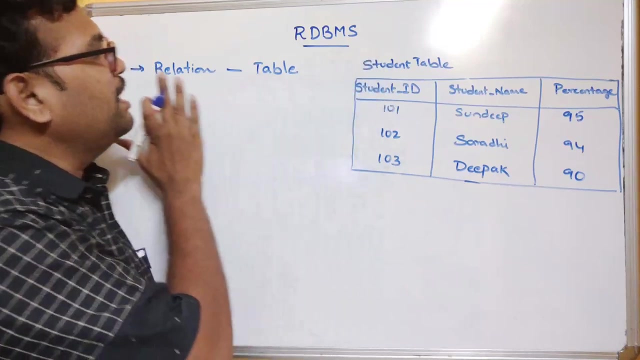 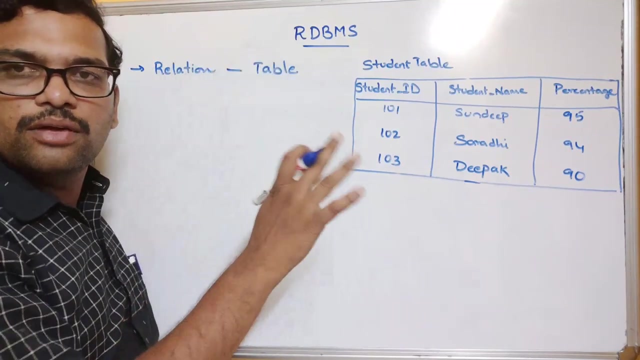 table, and this we call it as a relation in RDBMS. So here you can see, we are giving the student details. all the student details are being organized in a tabular format, So that's why we call it as a relation, right? So a relation means a table which consists of rows and columns and data, and 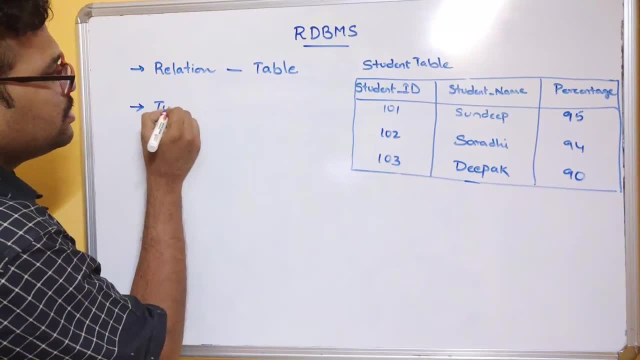 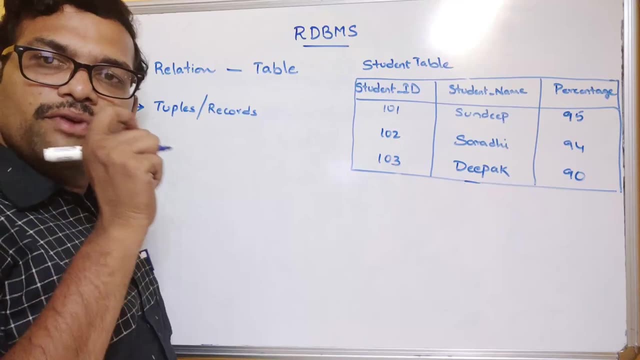 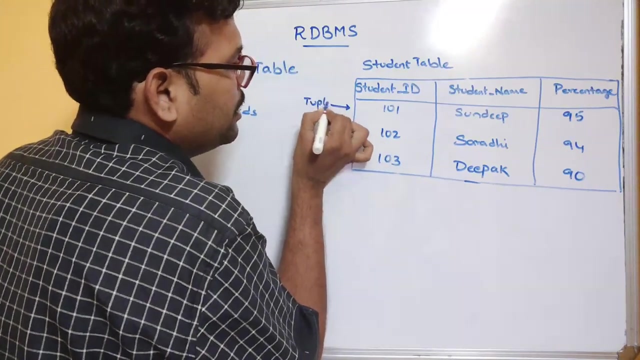 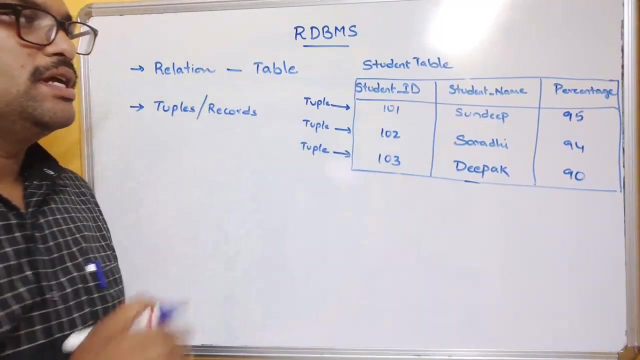 the second terminology is tuples or records. So the individual row is known as a tuple. So if you observe, so this is one tuple and this is another tuple and this is another tuple, or we can also call it as a records. So, for example, you can see here: So this particular row consists of the details of a. 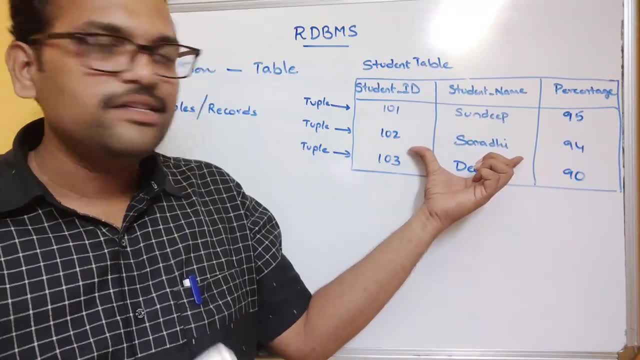 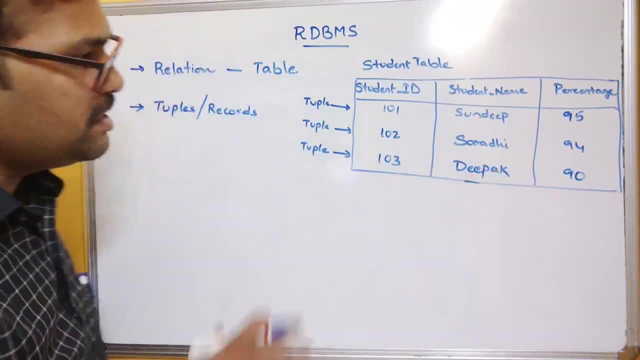 student suddenly. So, for example, you can see here. So this particular row consists of the details of a student suddenly. The second row consists of the details of a student suddenly. Third row consists of the student details related to Deepak right. So that means we are having the three rows. 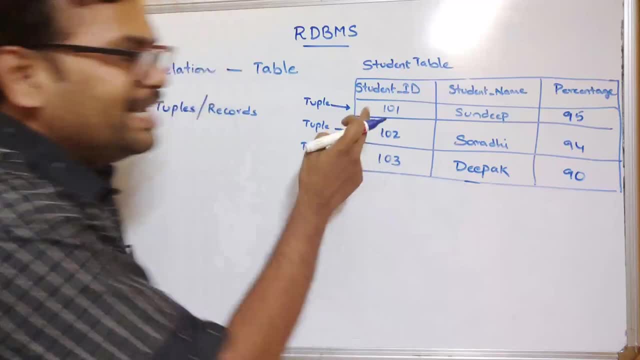 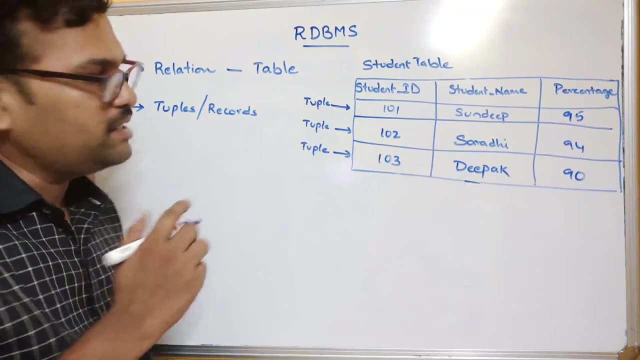 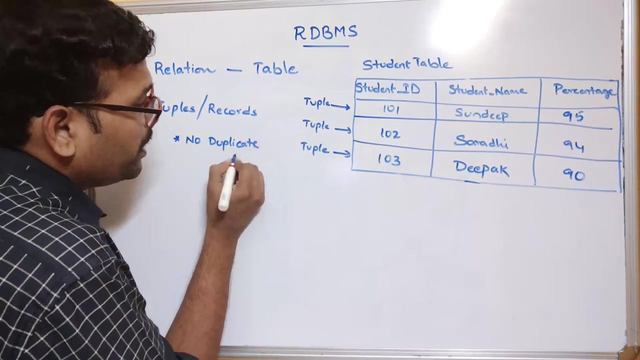 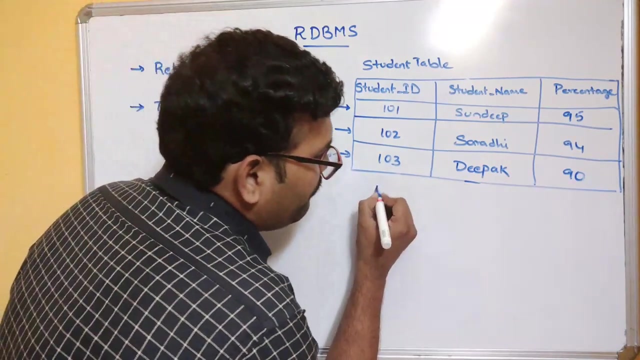 We are having some three student details. right, Each row is known as a tuple or record. So here we need to remember a few things. that is, in tuple there should be no duplicate values, no duplicate tuples. right, That means identical tuples should not be included in the relation. For example, we are having 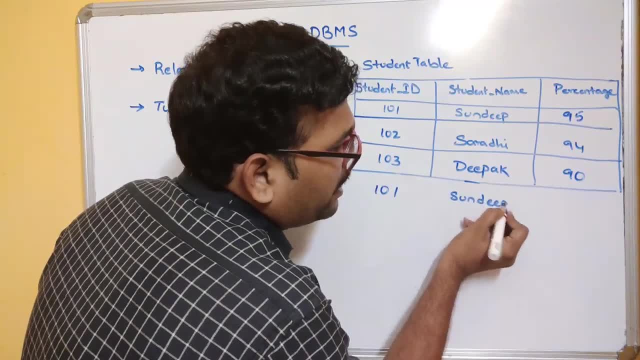 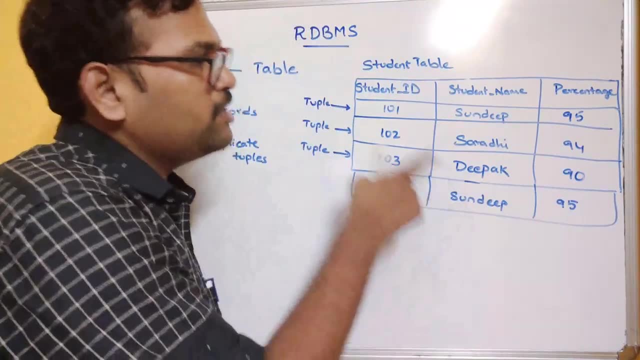 a fourth row, 101, and Sandeep and 95.. So if you observe here the fourth row, the fourth row is having the unique elements of the first row, So 101, Sandeep 95, 101, Sandeep, 95.. 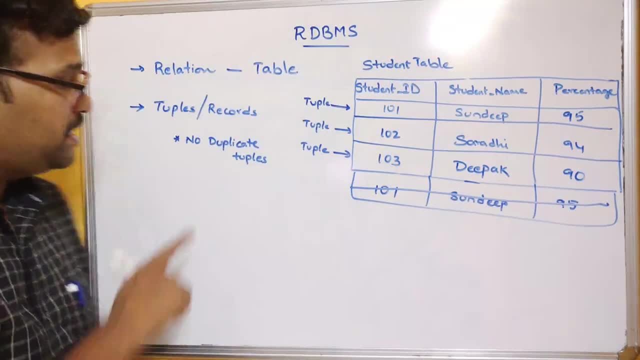 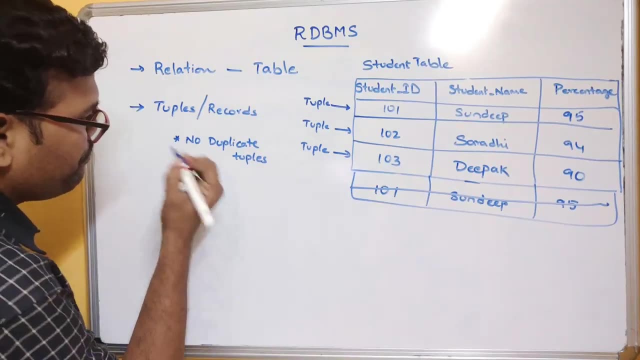 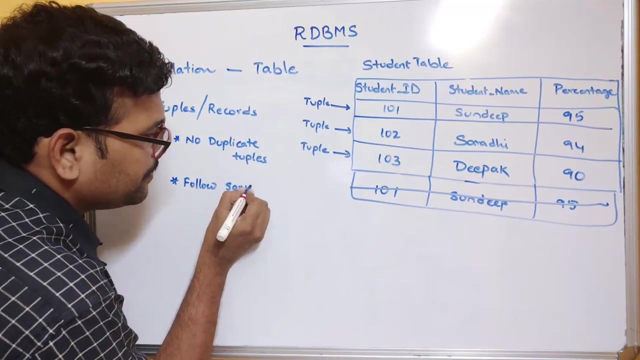 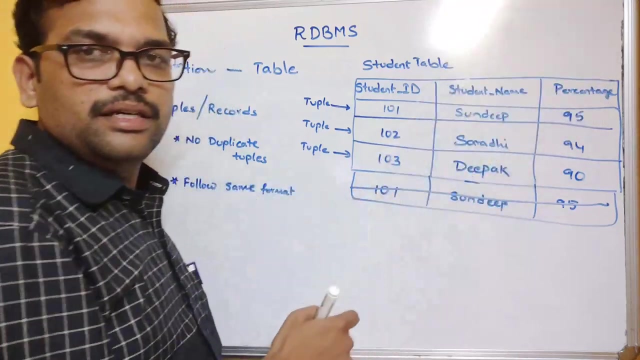 So this should not be accepted. That means no duplicate tuples should be available right. So this should not be accepted. That means no duplicate tuples should be available right. And so all the tuples should follow same format. same format: that means the first one- student ID, student name and percentage. So the same format should be followed for all the students, right. 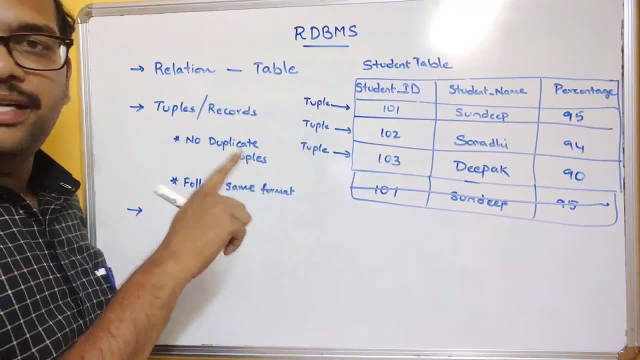 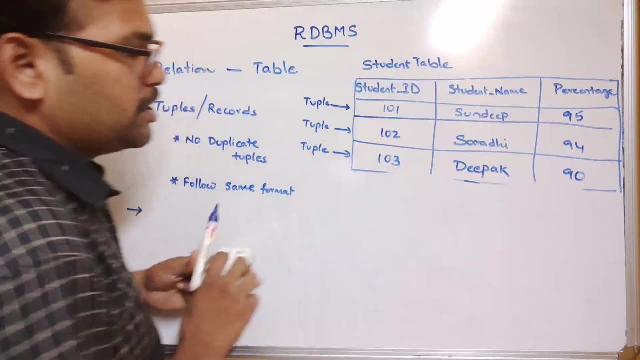 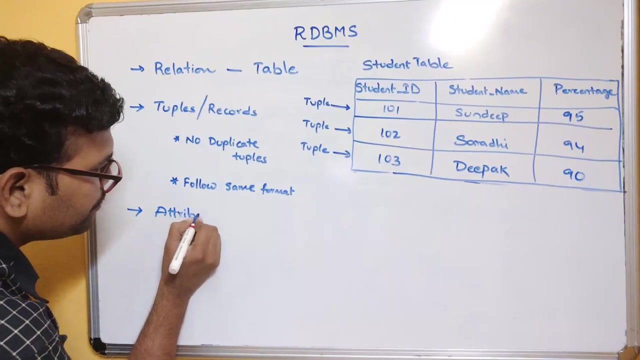 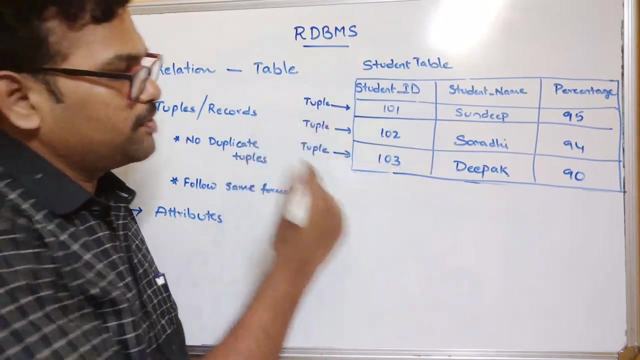 And the next terminology. so these are called as a tuples. right, these are called as a tuples And I am removing this one. So no duplicate should be allowed in tuples right Now. next one: attributes, attributes, And these attributes are known as the columns. okay, the columns. So this is an attribute. 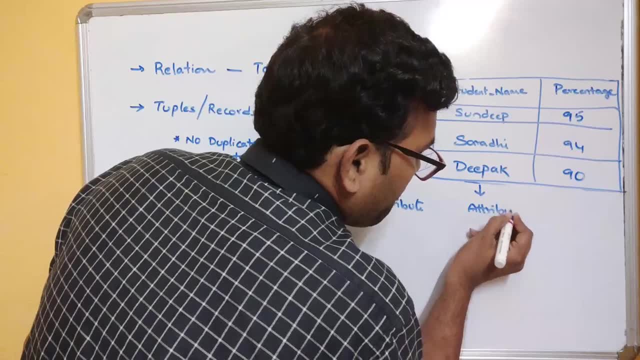 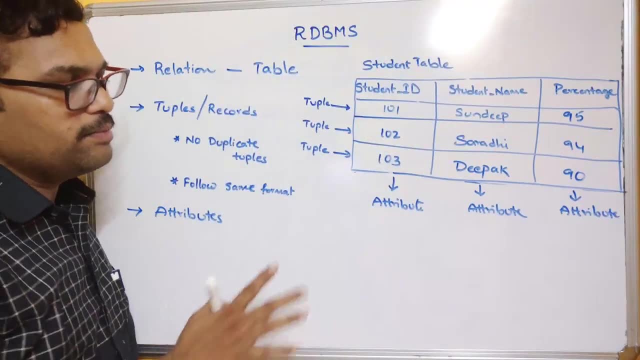 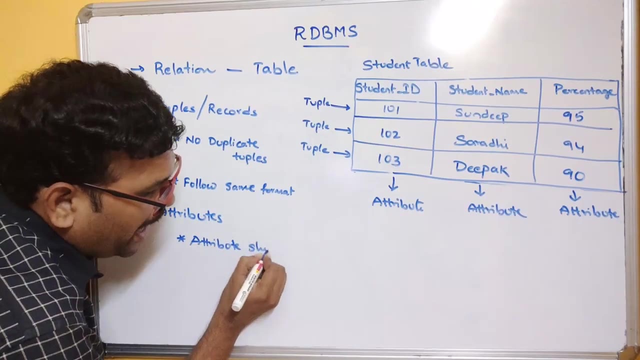 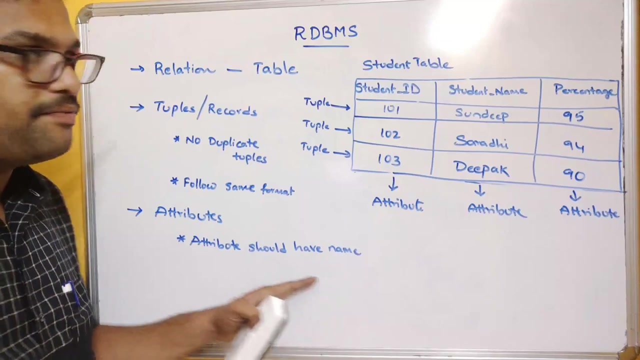 And this is an attribute. So attributes are for the tuples. So you can observe that rules are: first, attribute should have a name. Attribute should have a name to identify, to name should have a name to identify. So here, student ID is an attribute, Student name is an attribute. Percentage is an attribute. 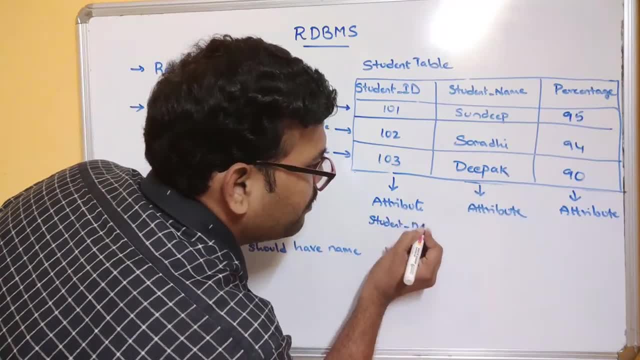 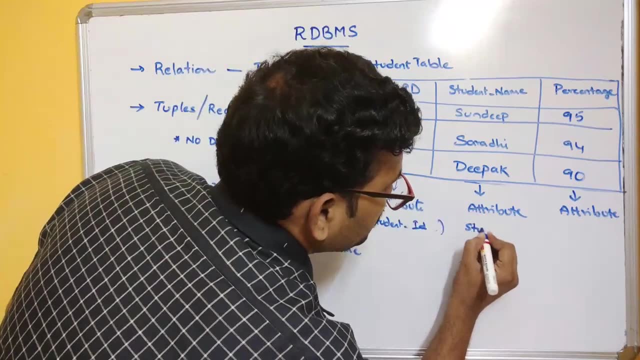 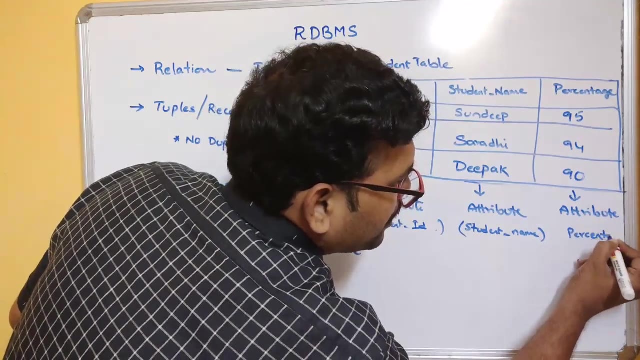 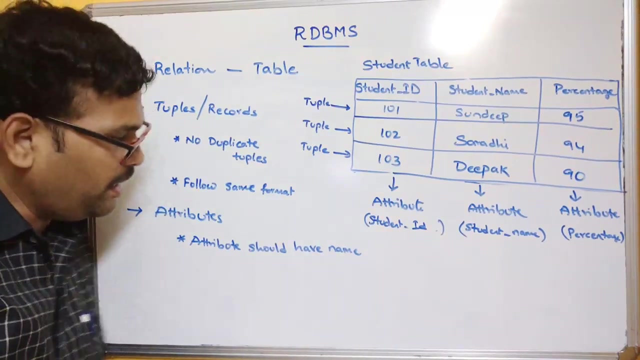 So here I am writing: student name is an attribute, Sorry, student ID. the first one is ID, Then student name is one more attribute, Percentage is one more attribute. So every attribute should have a name to identify right, And also there will be a unique attribute. 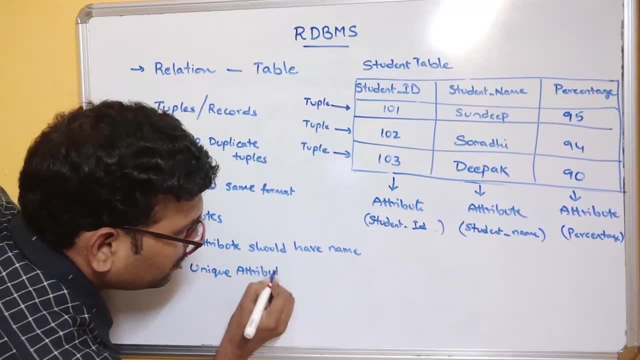 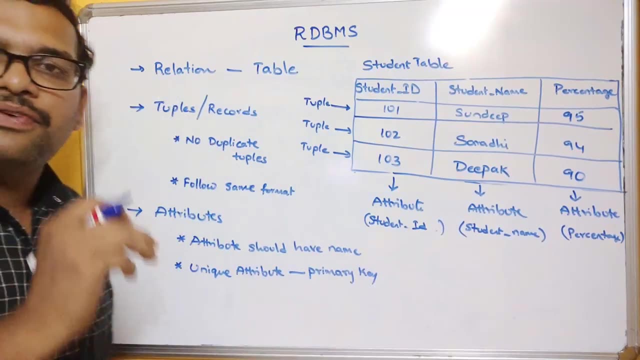 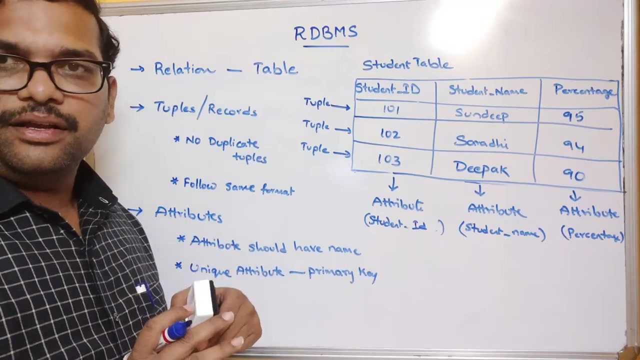 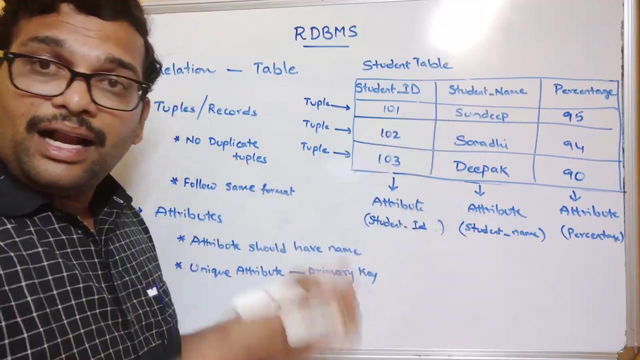 Unique attribute known as a primary key, Primary key to identify the tuples. okay, To identify the tuple, there should be a unique attribute called as a primary key, right, For example, if you take student name, so Sandeep, So in a class there can be multiple students with the same name. 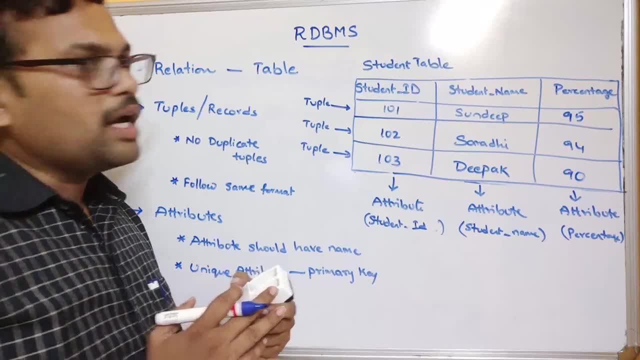 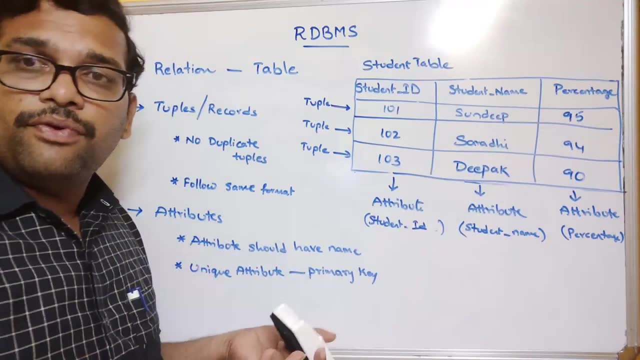 So it should not be considered as a primary key. Come to the percentage: So more than one student can get an equal percentage. So, for example, 94.. So 94 is a percentage which can be get for multiple students, right. 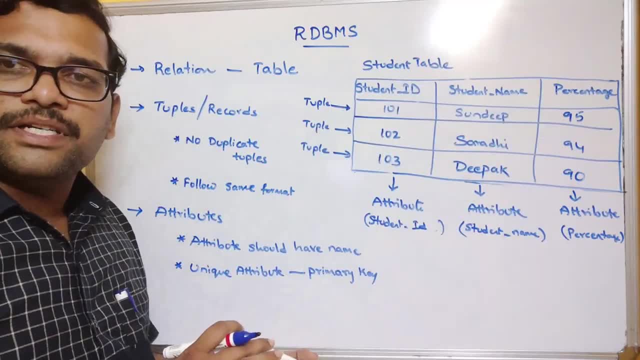 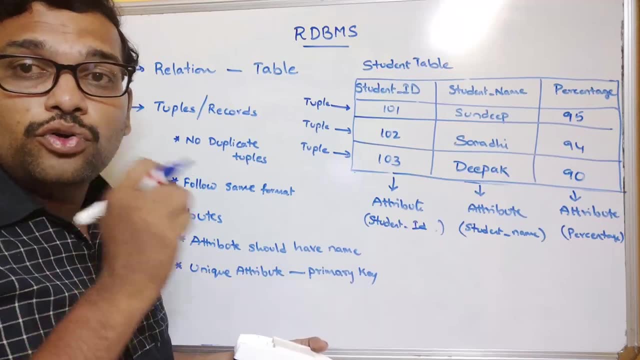 So there might be a chance. So that should not be considered as a percentage. So come into the student ID. So student ID will be the unit right. So no two students will share the same student ID. So such 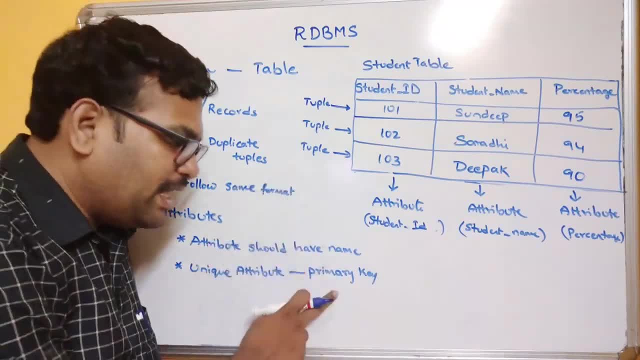 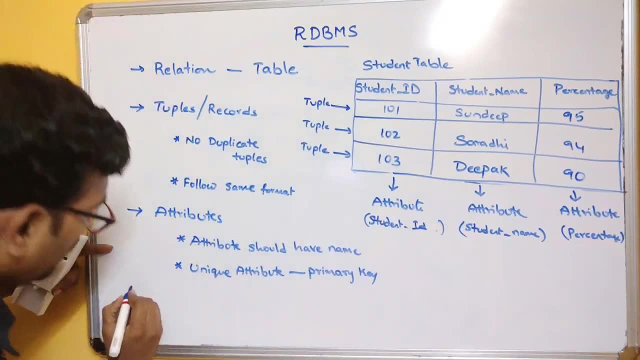 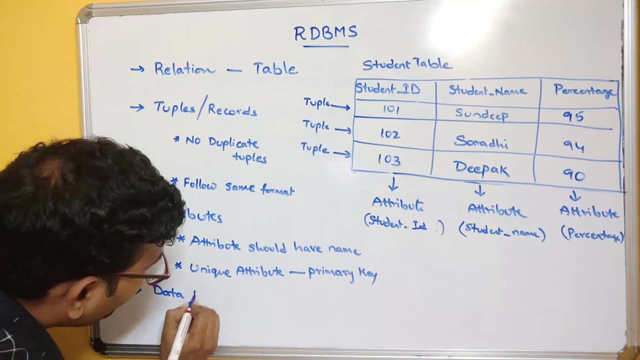 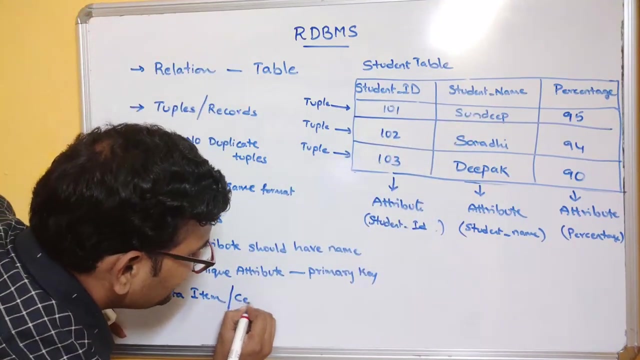 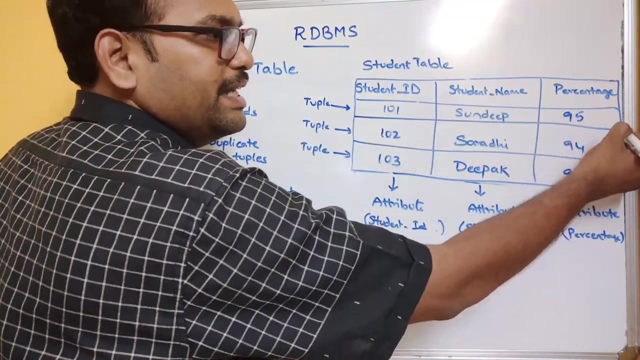 attribute. we call it as a unique attribute and that is, we call it as a primary key to identify the complete tuple right and the next one, data item. so data item means the actual data, so this is also called as cell data, cell data. so you can see, this is one cell, another cell, another cell. so these 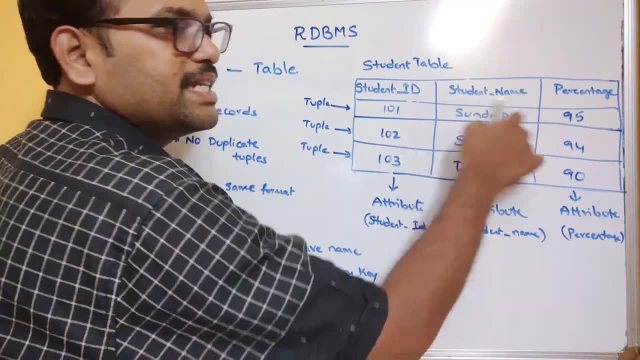 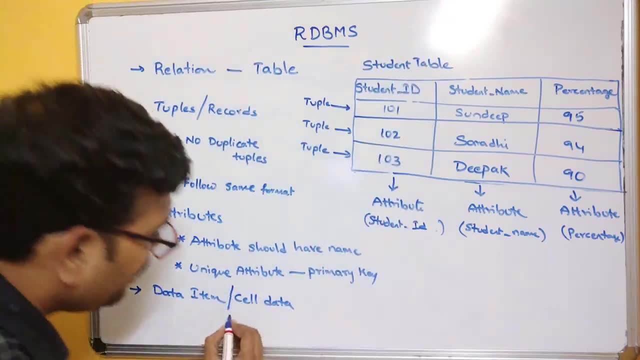 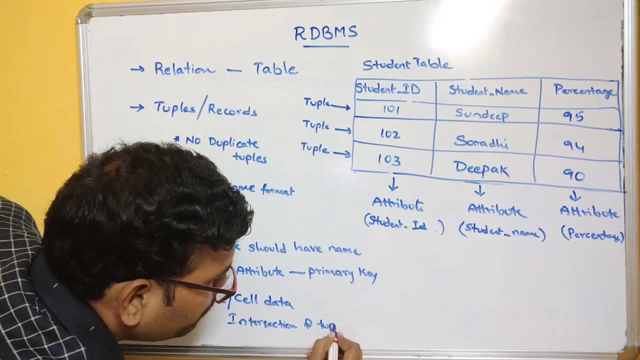 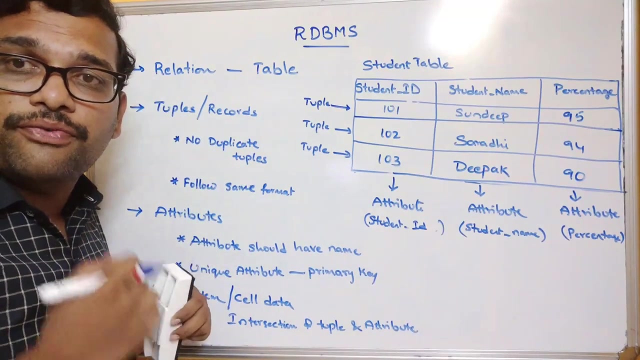 points we call it as a cells. these blocks we call it as a cells. so a cell is an intersection of a tuple and attribute. okay, cell is an intersection intersection of a tuple and attribute. so simply we can say it as intersection of row and column. so if you observe this one, it is an intersection. 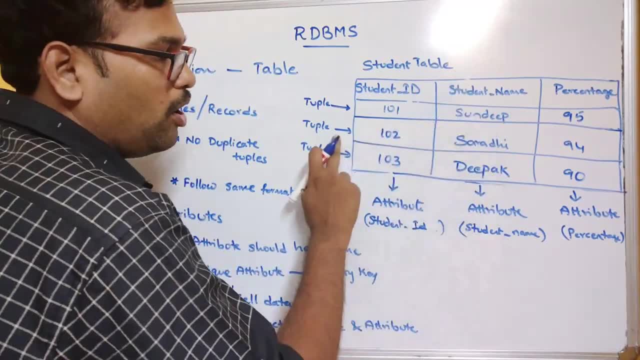 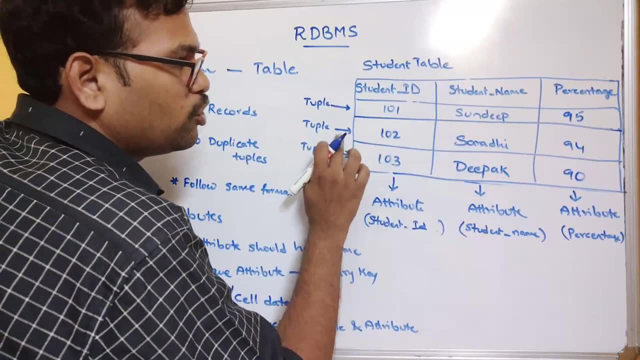 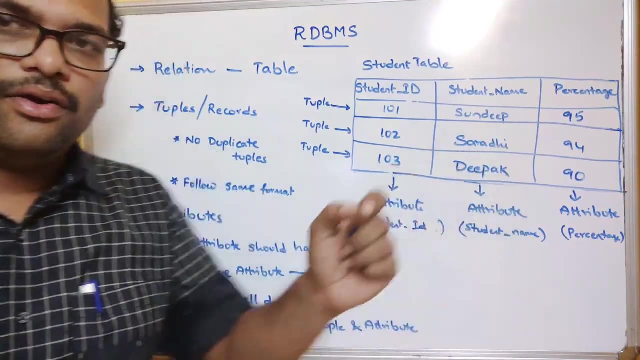 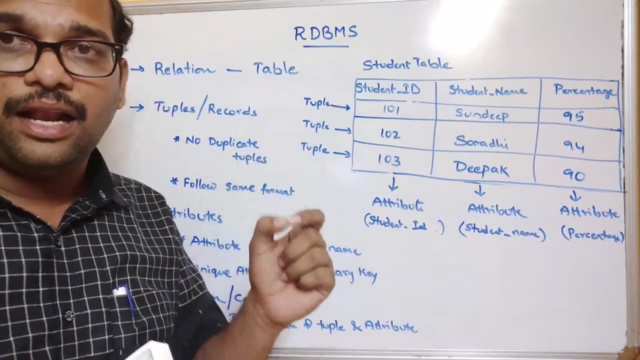 of tuple and column right, so horizontally, horizontal row right and a vertical column, so this will be represented as tuple and attribute intersection. and these data must be okay. this data must be atomic. atomic means it should have a single value. the data cell or data item should have a single 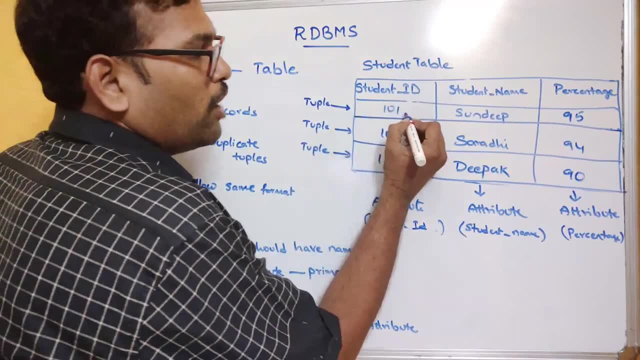 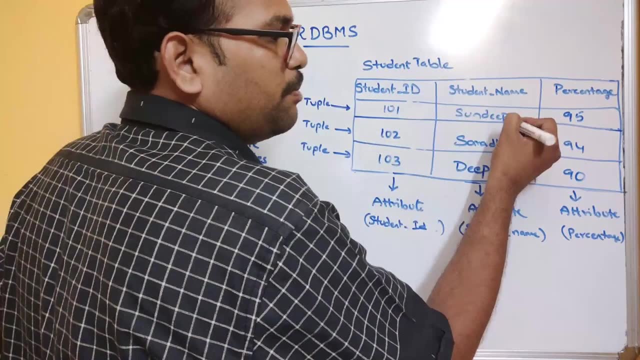 value right, for example student ID, so 101 comma 102. this is not a valid, so it should have only one value. so 101, so student name, Sandeep, comma ABC. so it is not a valid because it should have only one value. so the data, the cell data or a. 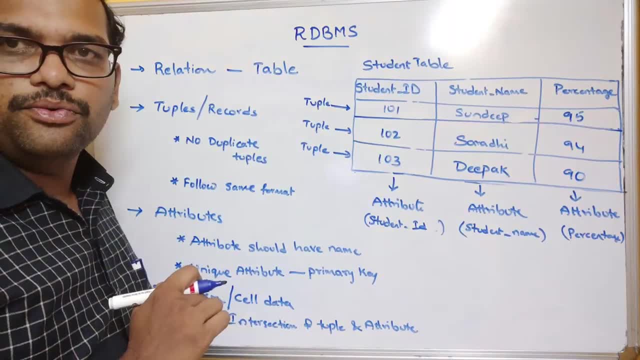 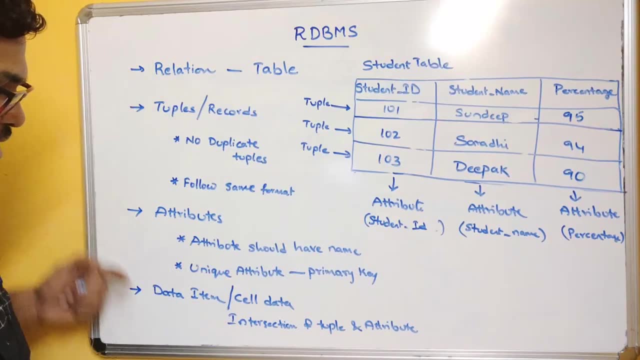 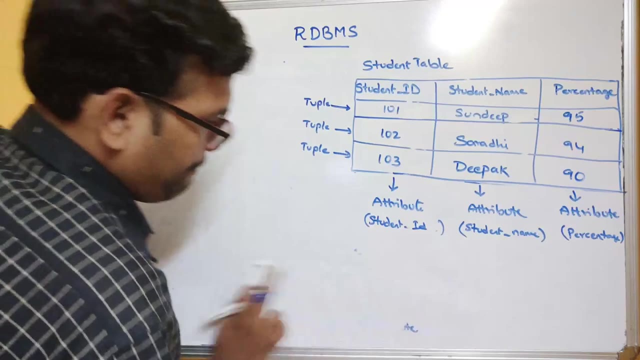 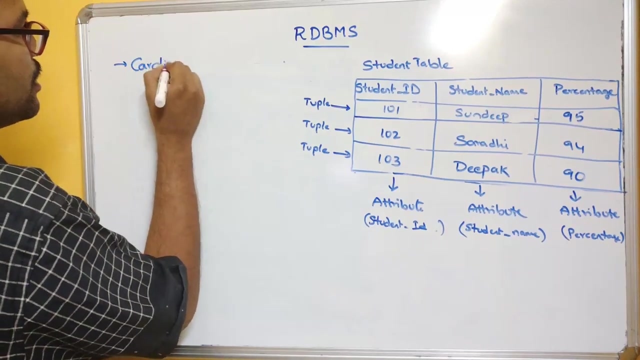 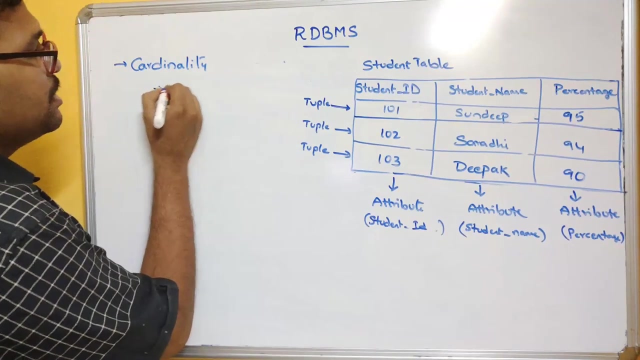 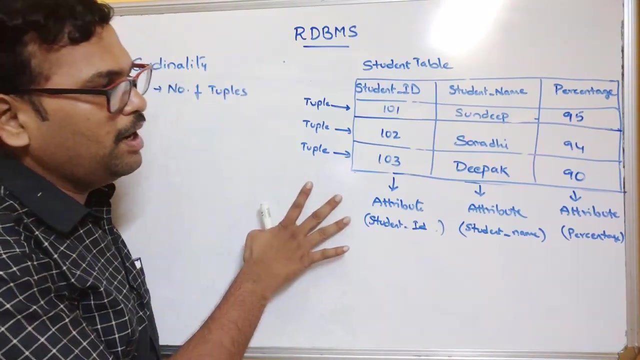 data item should have a single value, a single value, right? so relation: tuples attributes, data item. the next one, the next terminology is a cardinality, cardinality. so here the cardinality means a number of tuples, a number of tuples. a number of tuples gives the cardinality. so here, in this example, how many tuples are there? one? 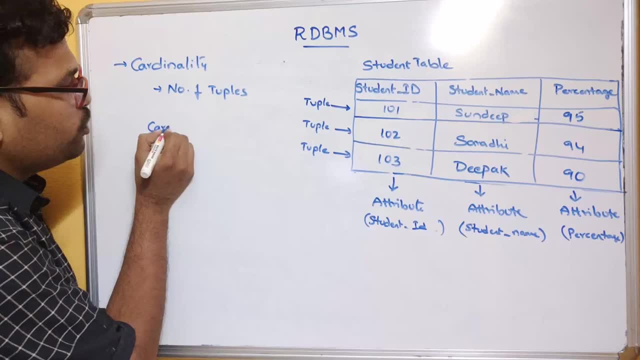 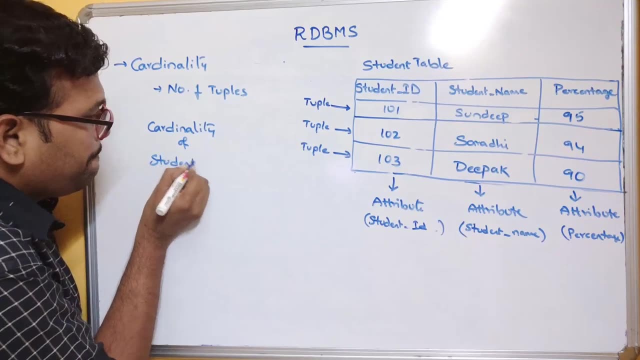 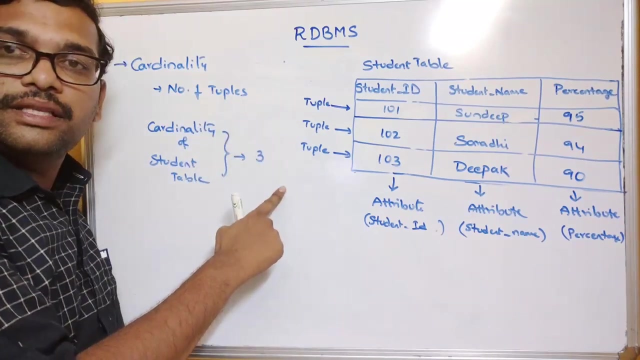 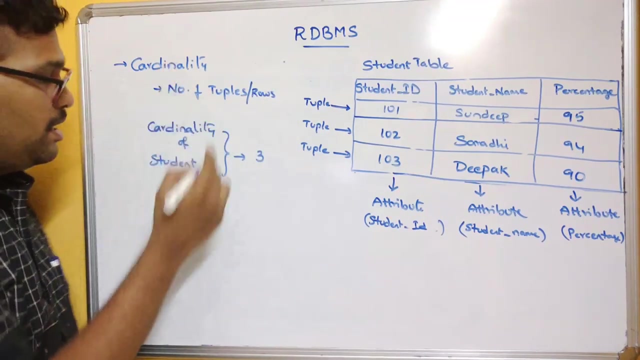 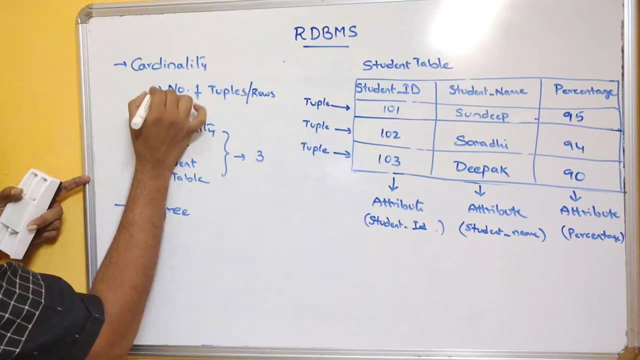 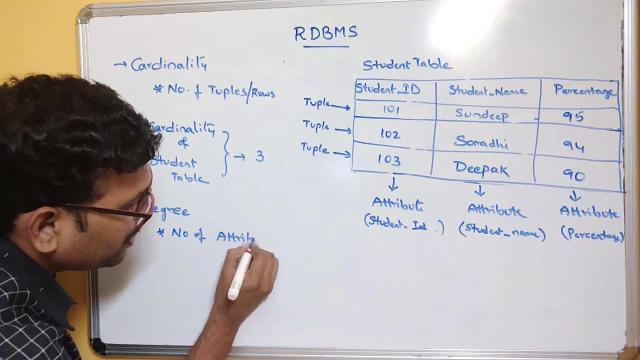 two and three. so the cardinality of the student table. cardinality of student table is three, because we are having the three tuples, three rows. so number of tuples, or number of rows, gives the cardinality. okay, the next one are degrees. so things, number of attributes, number of attributes gives the degree. so this is. 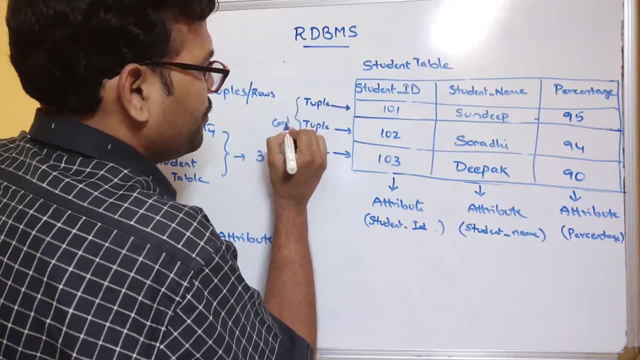 nothing but cardinality, and this is nothing but big right cardinality and is not to add 2, 4, 5, number 3, 4, 5, 4. this one is equal to Fig neiButey and this is nothing but a middle class deal, which indicates thatFr wag 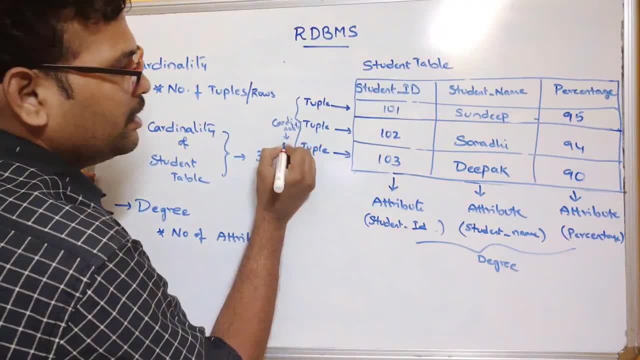 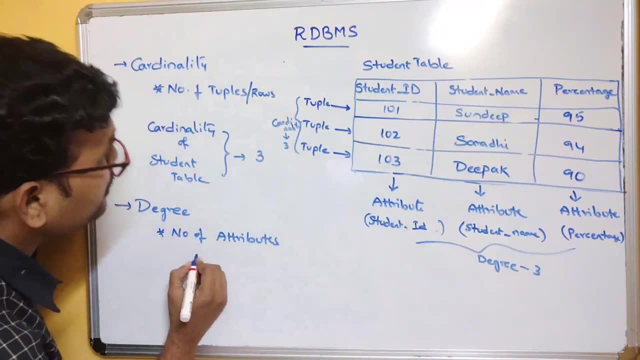 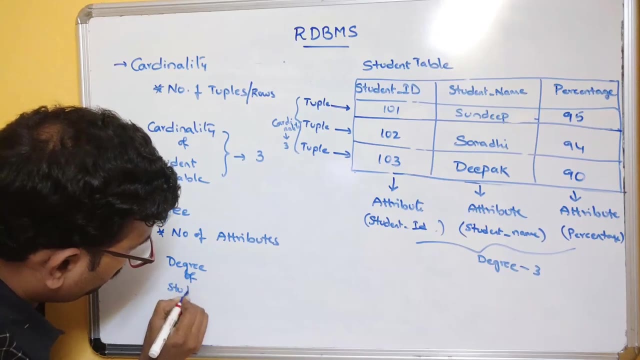 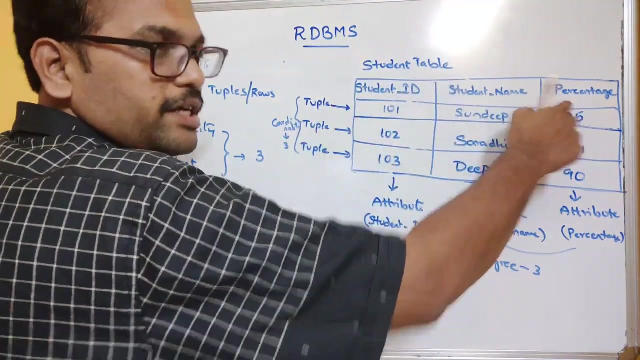 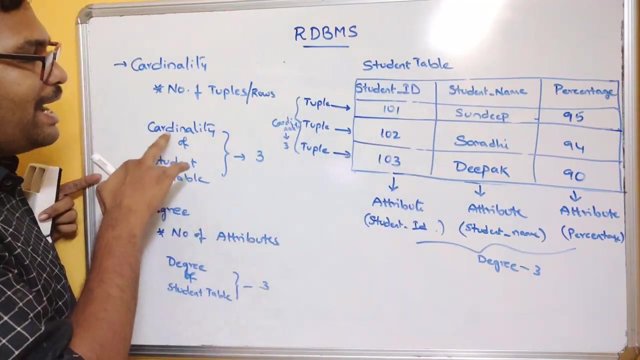 degree right, cardinality three. a degree three because number of attributes for the student table is a three. so degree of student table three because student id, student name and a percentage three attributes are there. that means the three columns right. so the degree of student table will be three. cardinality it's a number of tuples or number of rows or number of records. the next one. 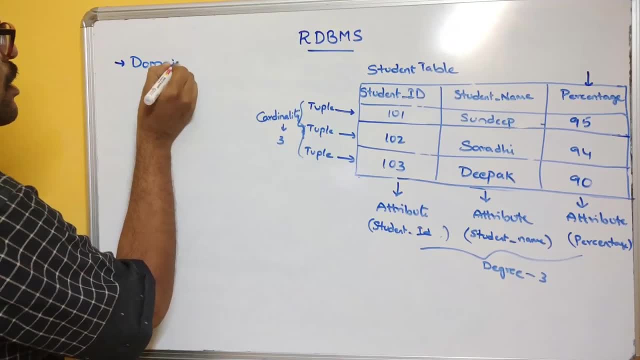 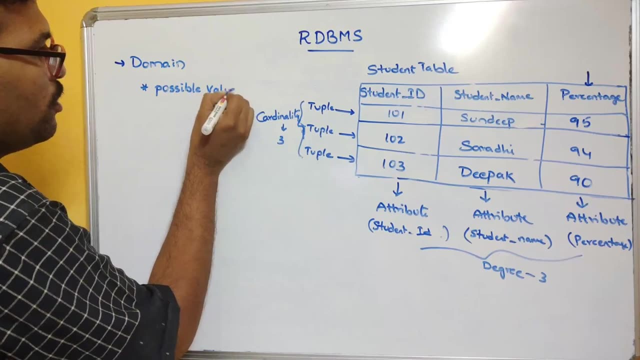 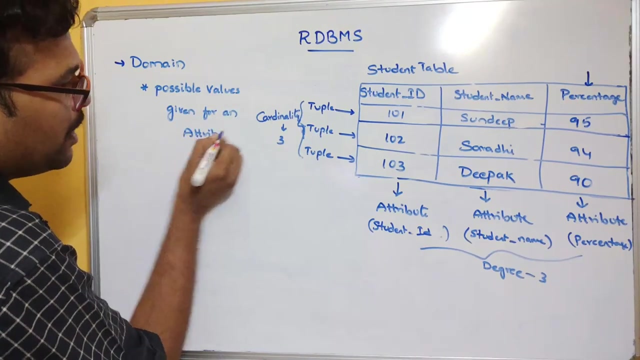 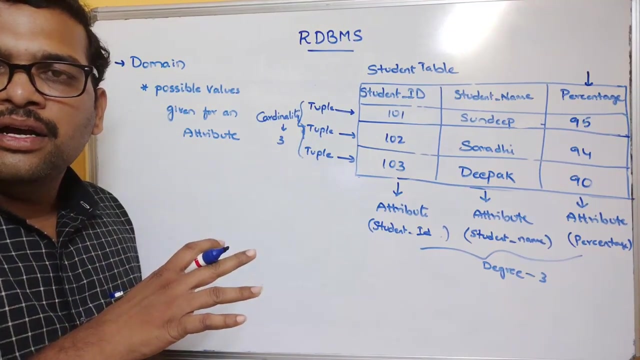 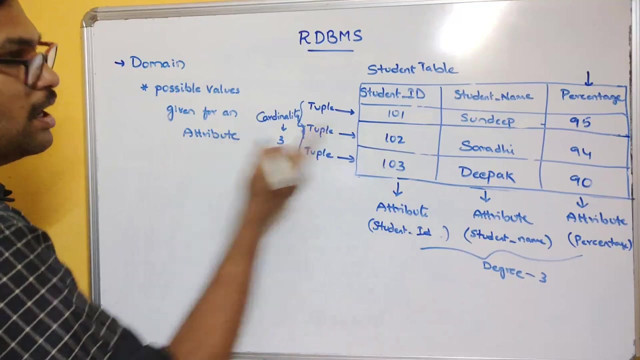 is domain. so domain means all the possible values given for an attribute. so attribute is a column. so we need, we are supposed to give a value for an attribute, right? so what are the possible values that should be given, for an attribute is called a domain in this example. consider this percentage. so percentage will be zero to hundred in between. 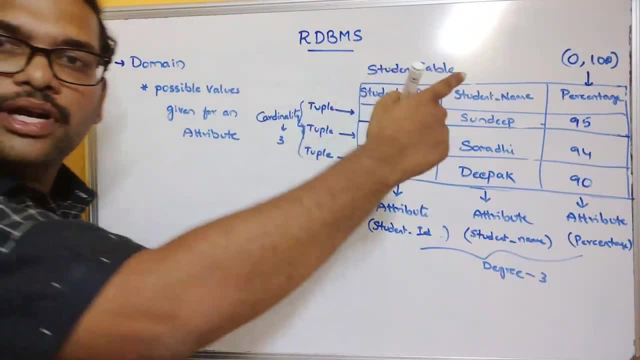 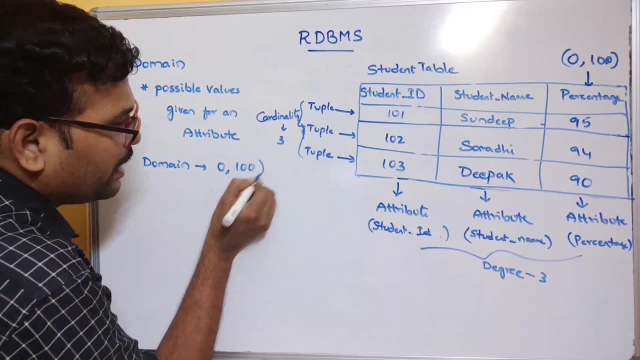 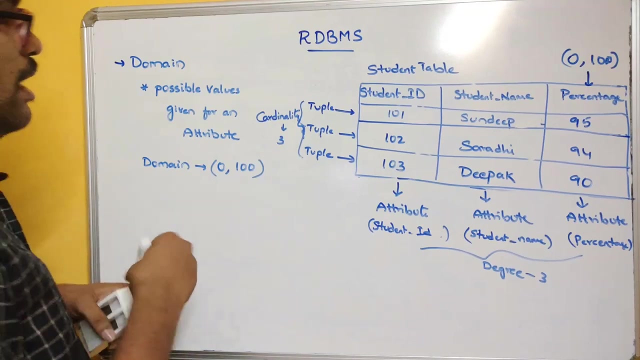 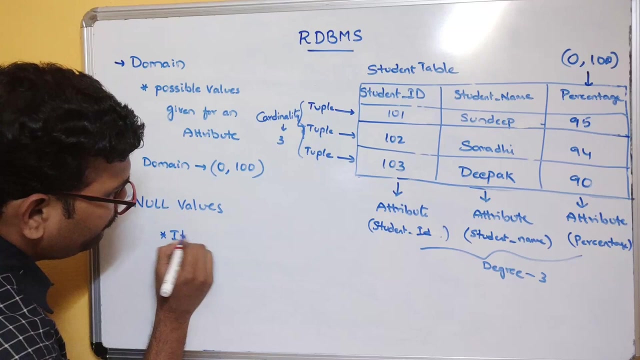 zero and hundred right, so that is called a domain. so here the domain for a percentage is zero to hundred, so this is called a domain. right. the possible values given for the attribute. and the last one is a null values, null values. so coming to this, null values if a cell kept blank. 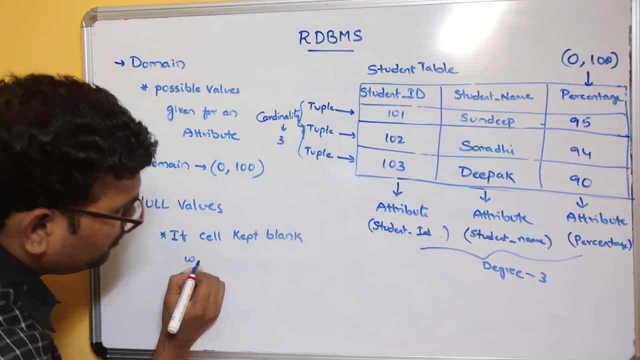 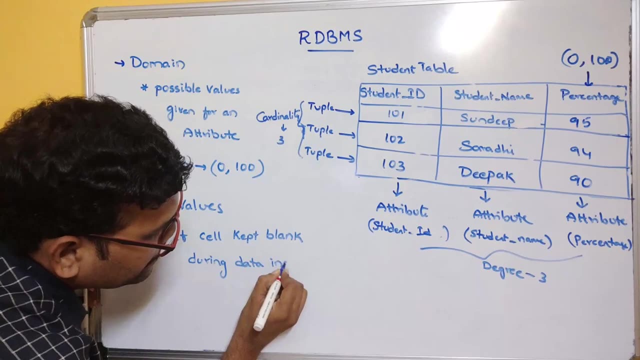 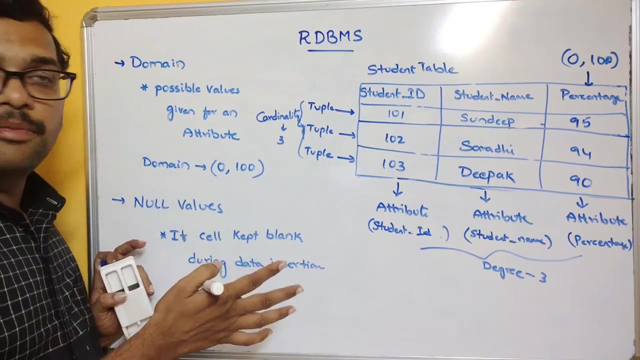 if a cell kept blank. if a cell kept blank During a data insertion, then that particular cell will be given as a null value. cell or attribute, whatever it may be, For example, the student ID 101, Sandeep, and if I am not giving this percentage right, 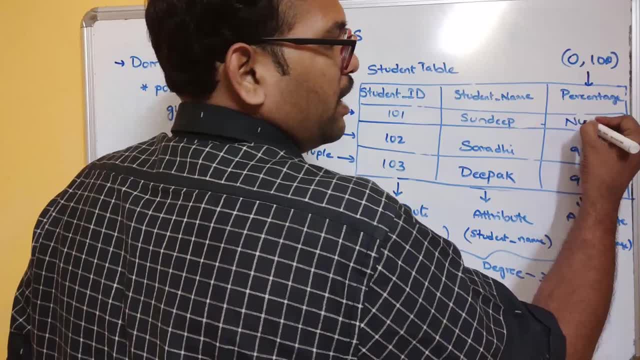 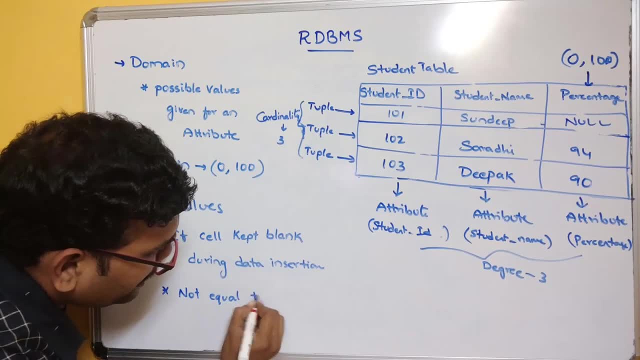 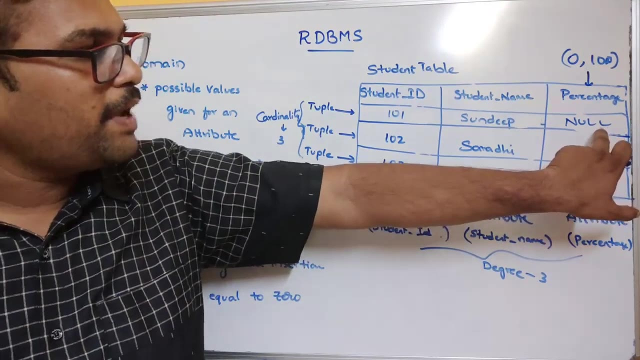 I just kept blank. then it will be filled with a null value. So this is not equal to, not equal to zero, right. So null, the null means that doesn't implies that the percentage is zero, right. So that percentage cell has been left blank, right. 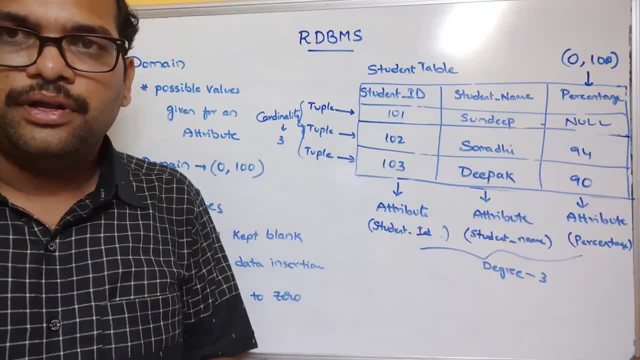 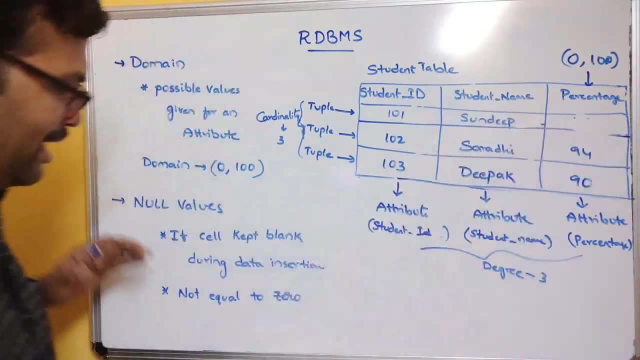 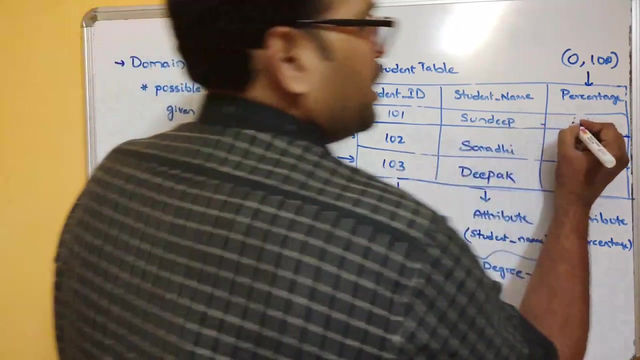 So we can fill that percentage in future. So at present that cell has been kept left. okay, So a null value. So null value means if any cell or an attribute kept blank during the data insertion, that blank will be represented with a null. 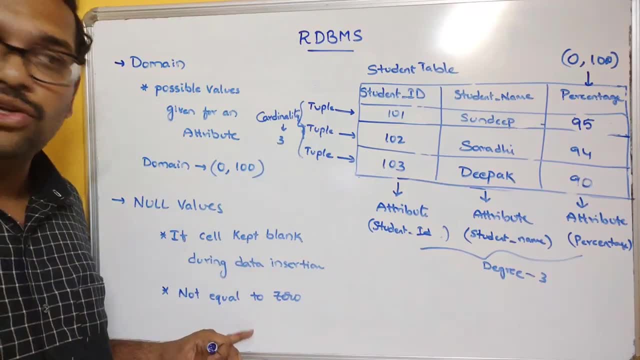 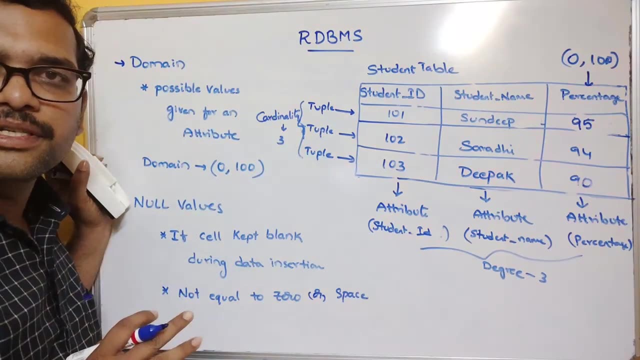 That blank will be represented with a null And this is not equal to zero or a space or any space. right, It's not equal to zero or any space. So this is the null values. So I hope you understood the basic terminologies of RDBMS. 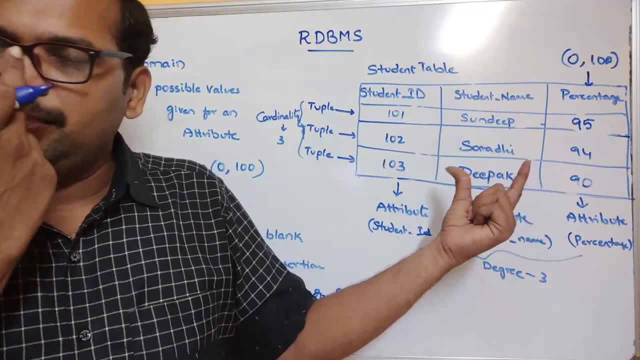 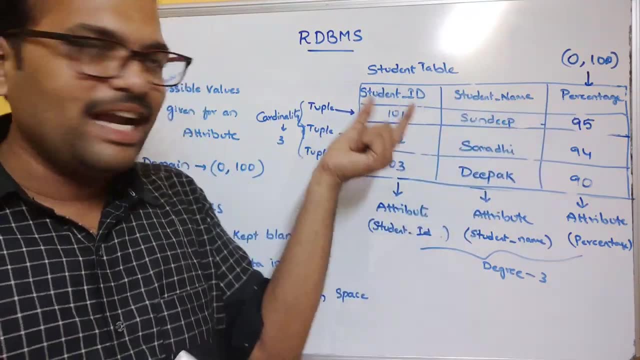 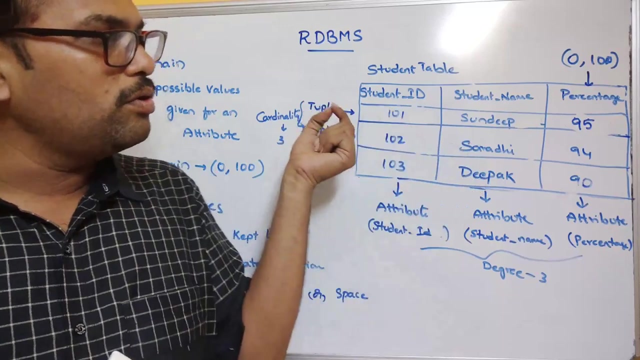 So this is called a relation, The table is called as a relation And the rows are called as a tuples, or records, And the columns we call it as a attributes, And each attribute we should have the name And unique attributes should be represented with a primary key in order to represent the complete tuple. 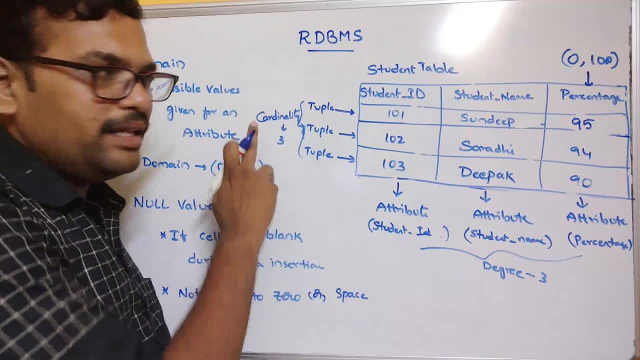 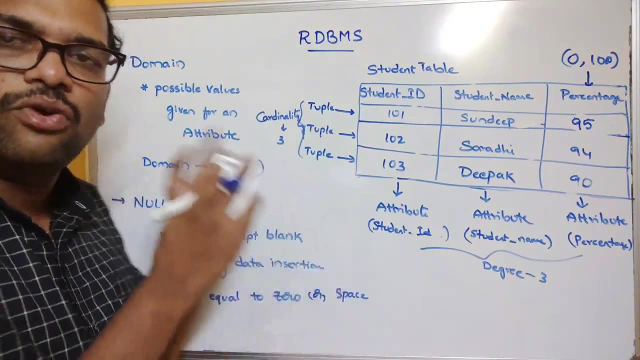 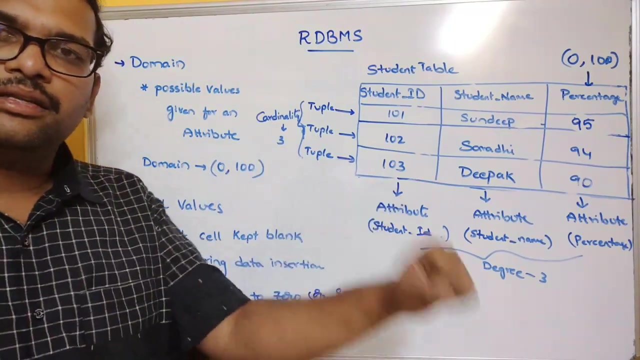 And the number of tuples, we call it as a cardinality. The number of columns, we call it as a degree And domain. the possible values given for an attribute is called a domain And null values. If the cell is kept blank during the data insertion, that particular cell will be filled with the null values. 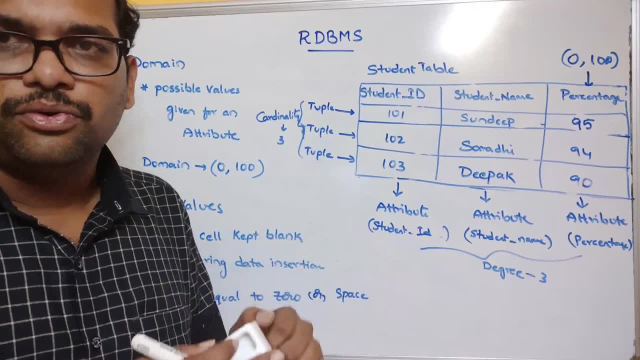 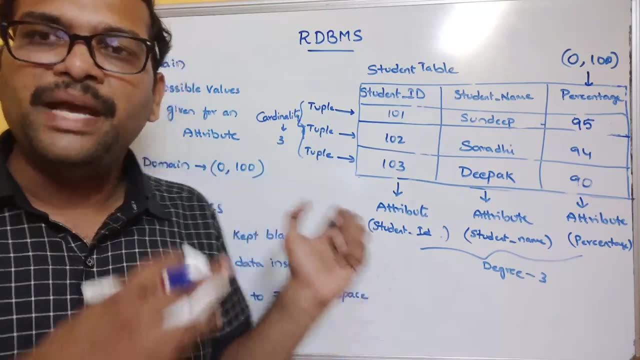 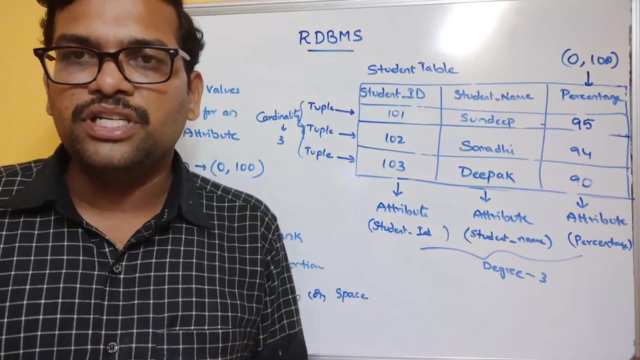 And it doesn't mean it is equal to zero or a space, right? So this is the basic introduction to RDBMS and the basic terminologies used in the relational database management system, right? So hope you understood this one, And if you are having any doubts regarding this one, feel free to post your doubts in the comment section. 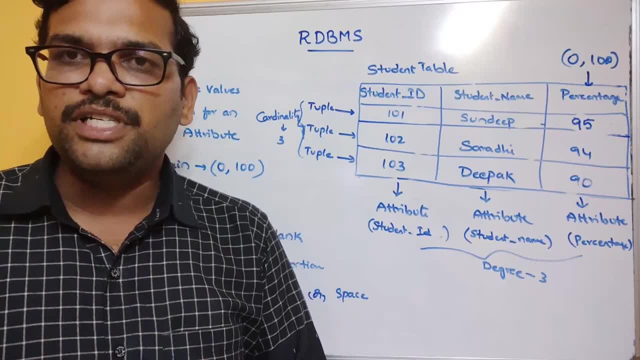 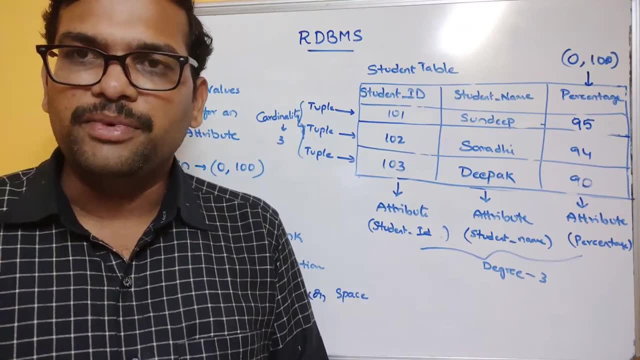 Definitely, I will try to Clarify all your doubts. If you really enjoyed my session, like my session, share my session with your friends And don't forget to subscribe to our channel. Thanks for watching. Thank you very much.